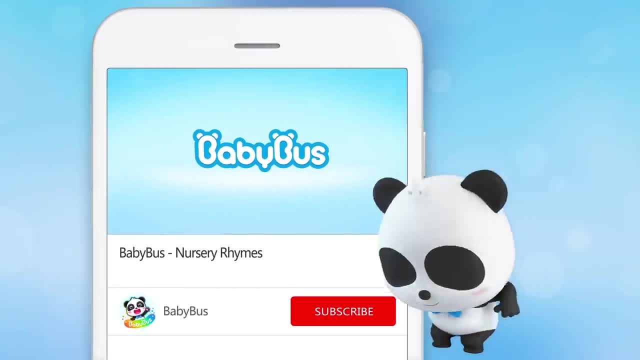 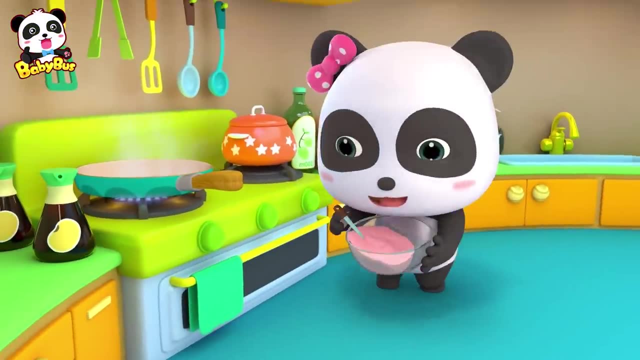 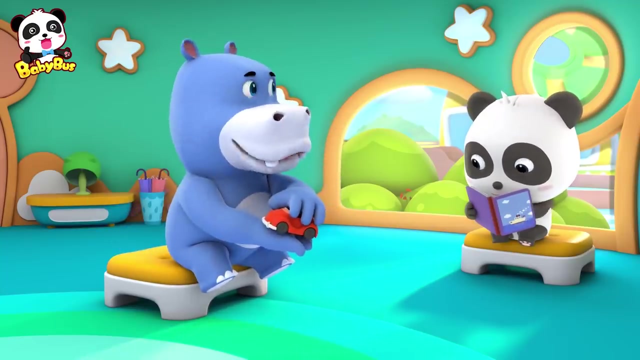 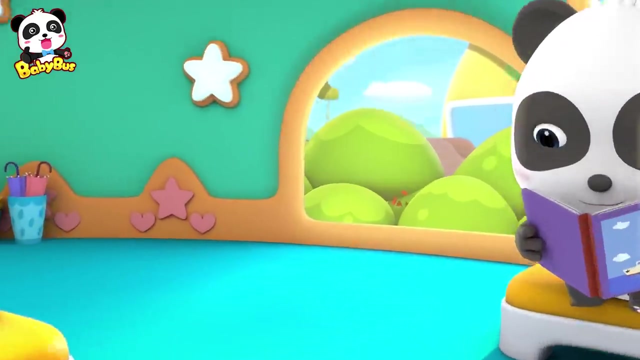 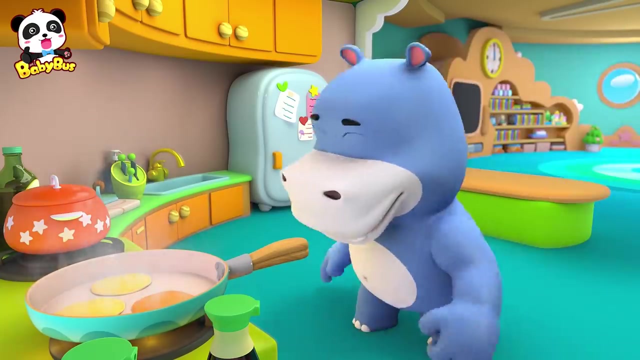 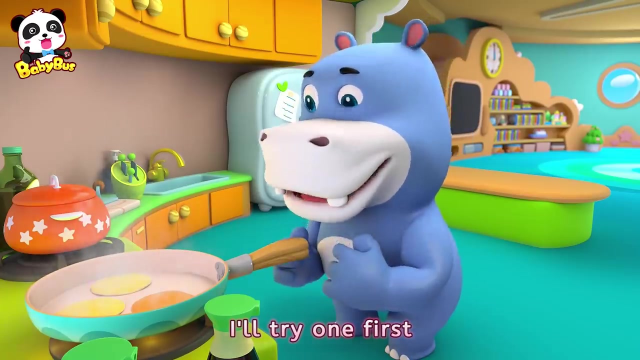 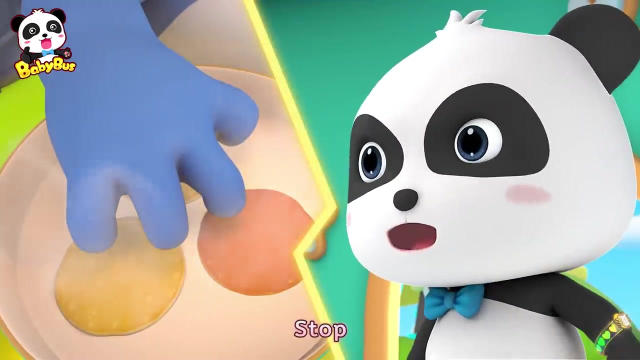 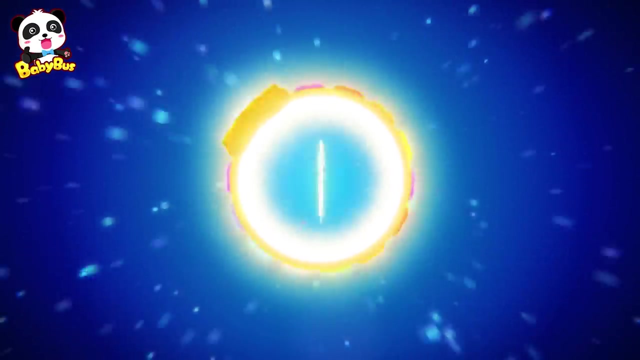 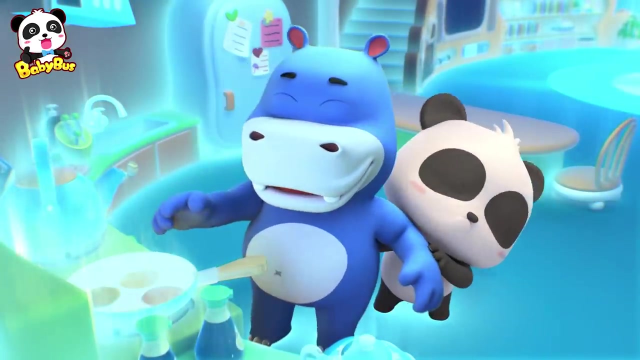 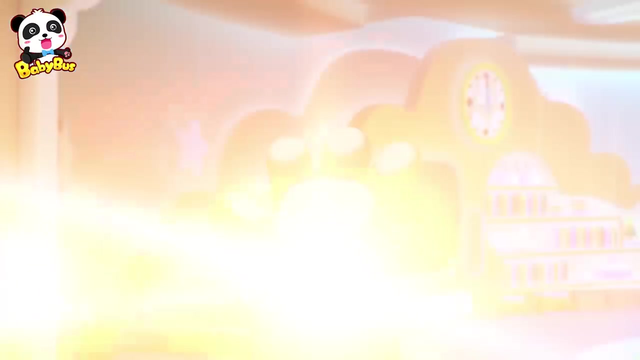 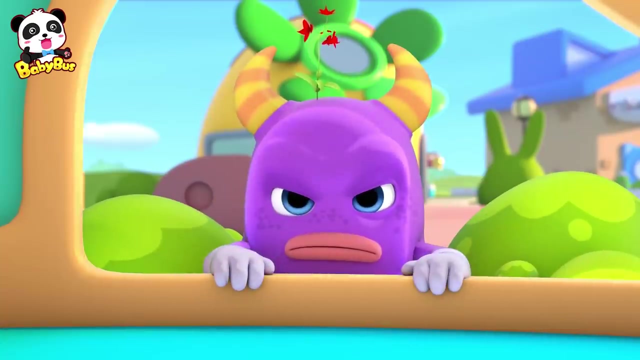 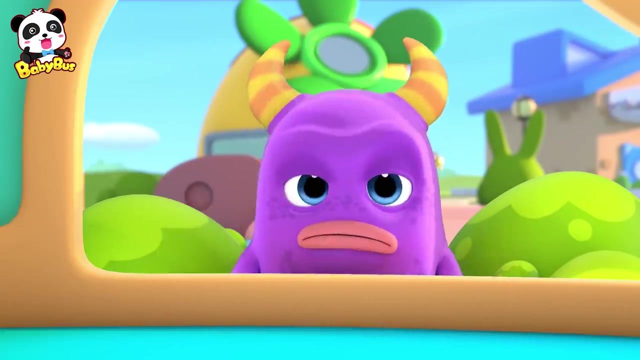 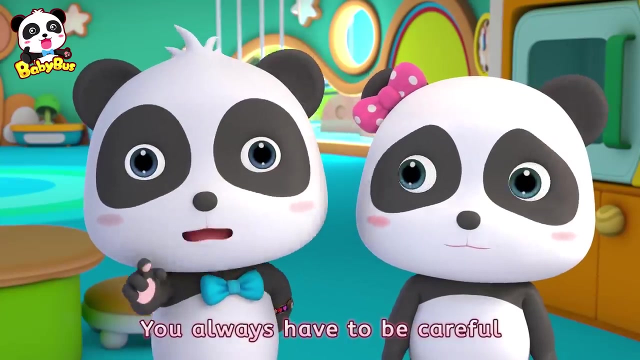 Baby bus. click here to subscribe. What's that smell? well, it smells great Dangerous coming. Wow, they look so yummy. I'll try one first. Oh, Nobody's in danger. I don't like it. Hey, you could have been really hurt. You always have to be careful in the kitchen. 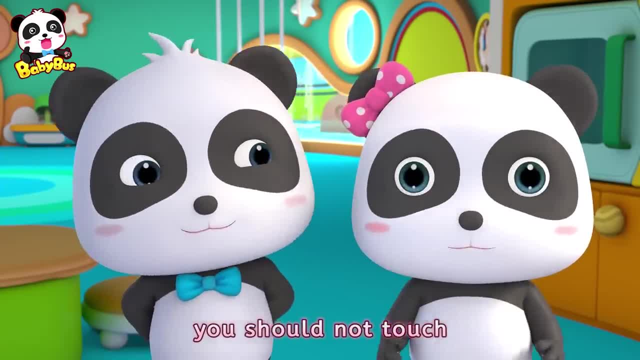 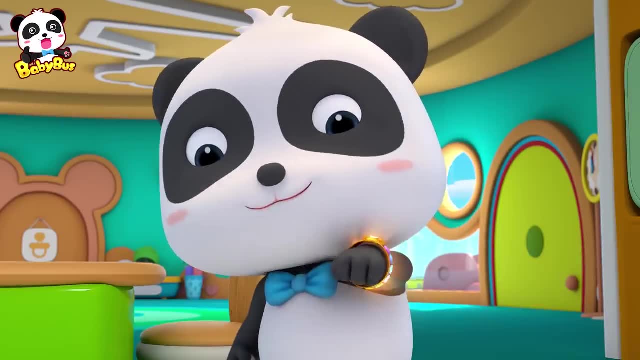 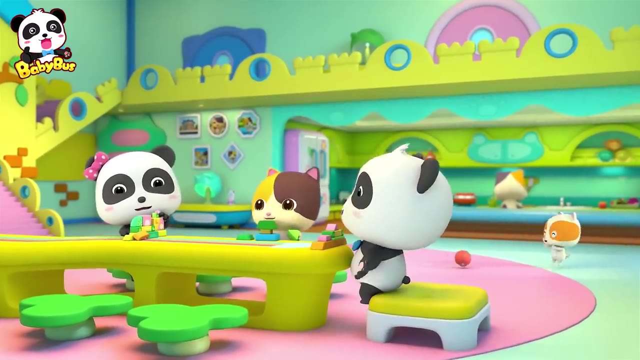 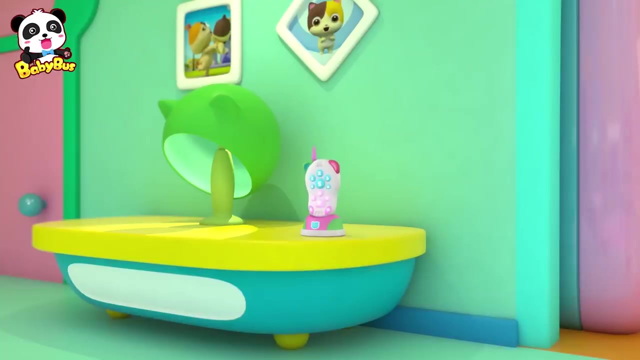 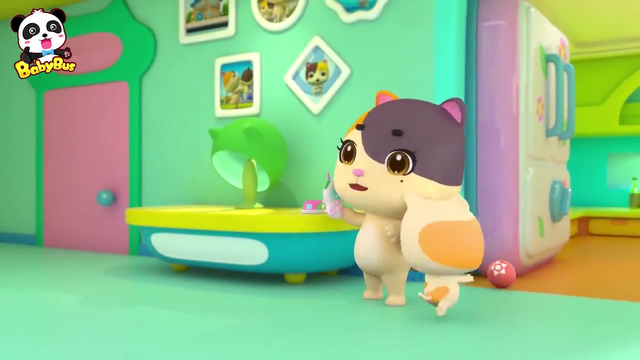 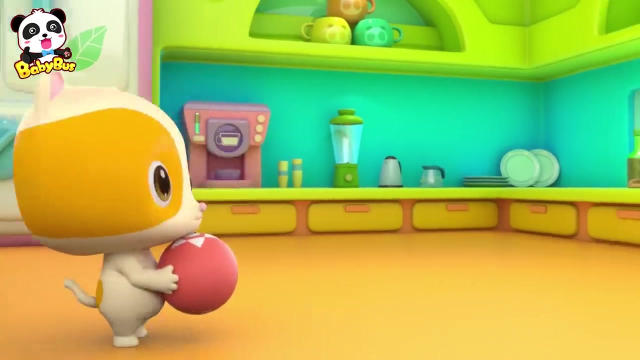 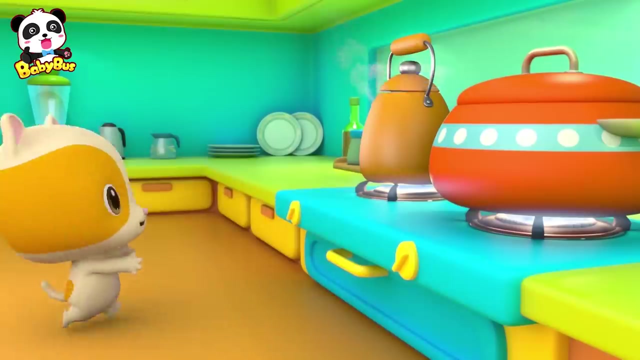 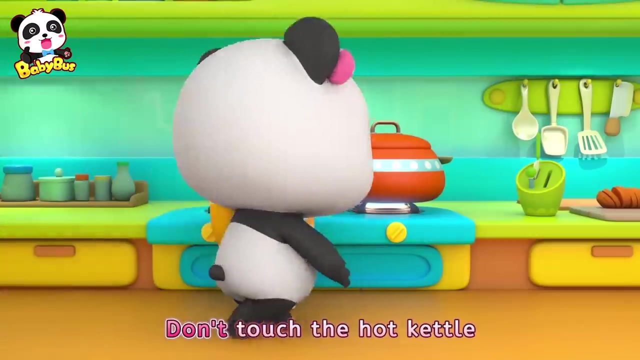 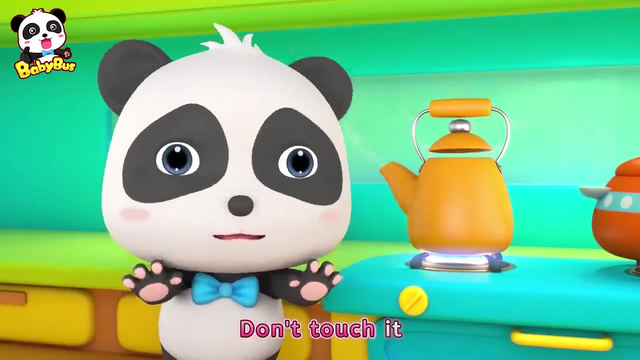 And there are many things you should not touch. What kind of things, for example, let's take a look: Hello, oh hi, All right, Wow, Don't touch the hot kettle, don't touch it, Don't touch, don't touch the hot kettle, don't touch it. 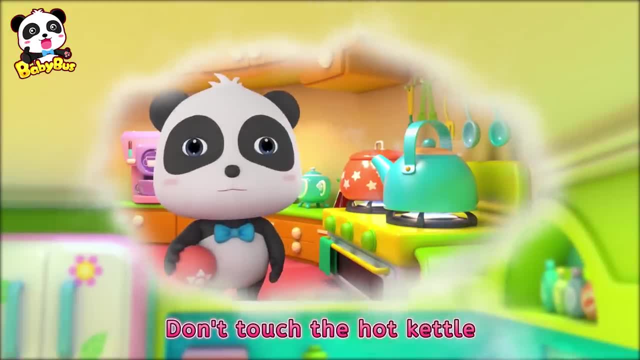 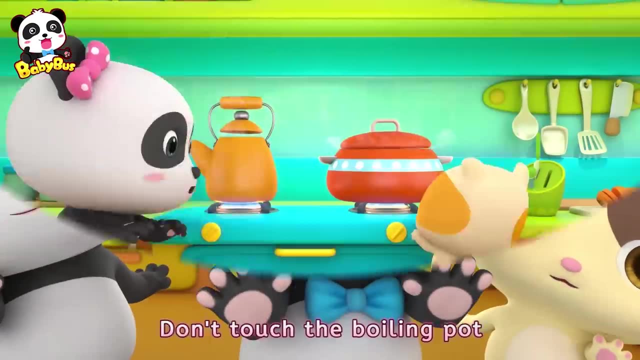 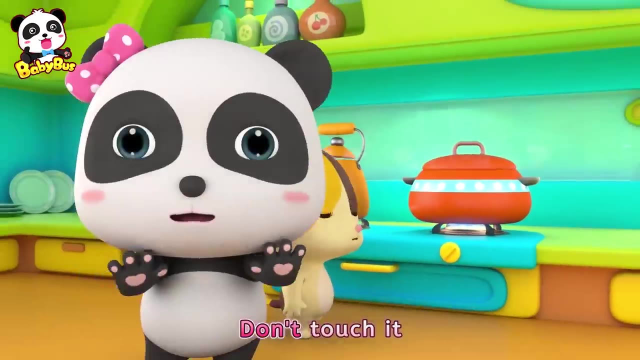 Don't touch the hot kettle. don't touch the hot kettle, don't touch it. it's dangerous. don't touch it, don't touch. Don't touch the boiling pot. don't touch it, don't touch. Don't touch the boiling pot. don't touch it, don't touch. 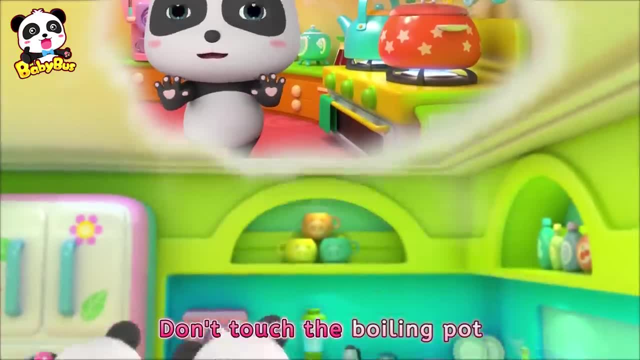 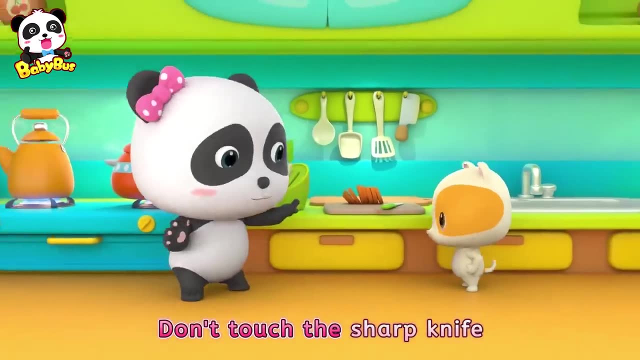 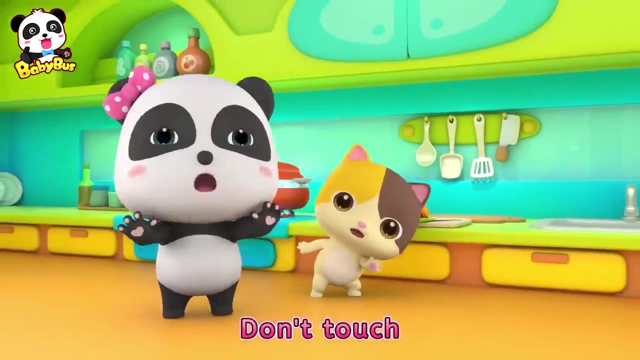 Don't touch the boiling pot. don't touch the boiling pot, don't touch it. it's dangerous. don't touch it, don't touch. Don't touch the sharp knife. don't touch it, don't touch. Don't touch the sharp knife. don't touch it, don't touch. 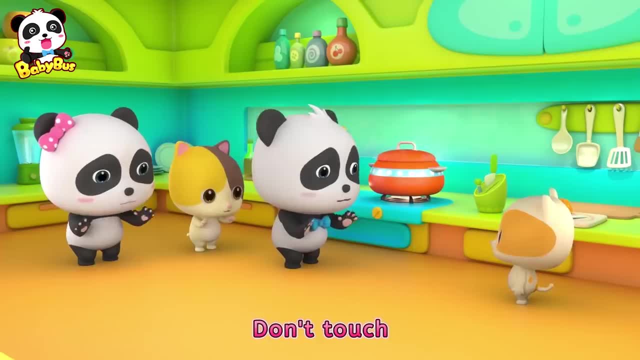 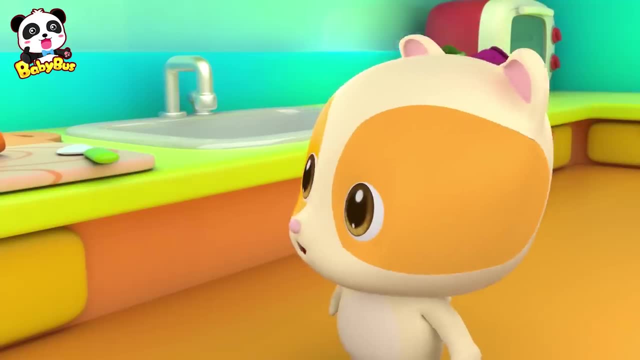 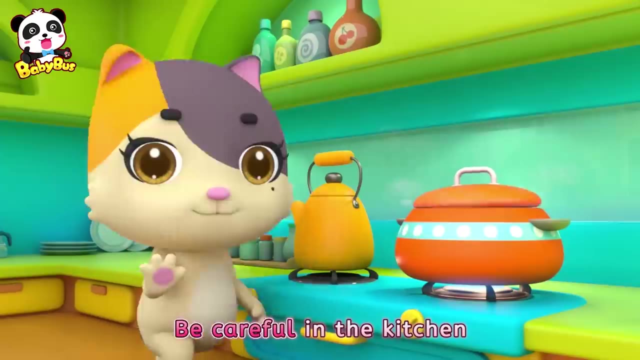 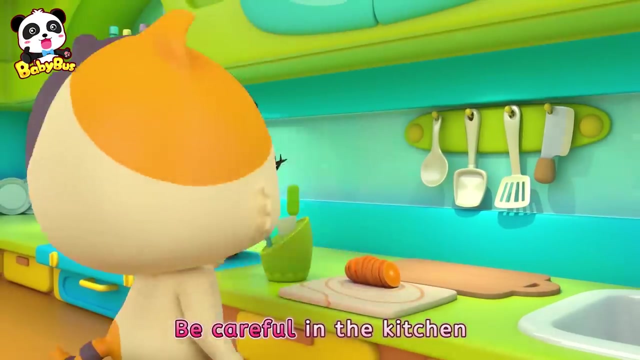 It's dangerous. don't touch it. don't touch Timmy. you shouldn't play in the kitchen. It's so dangerous. Be careful in the kitchen, be careful. Be careful in the kitchen, be careful. Be careful in the kitchen, be careful. 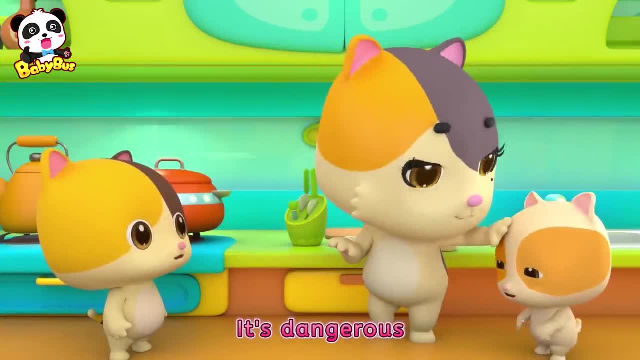 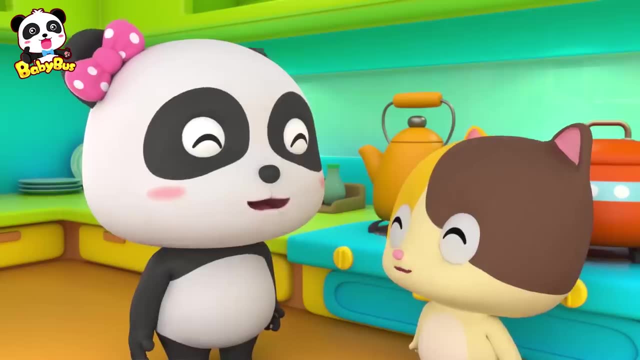 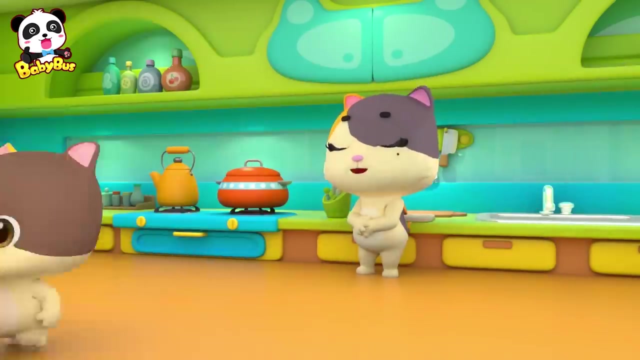 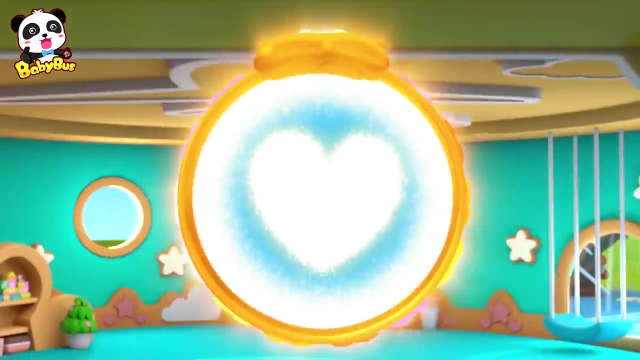 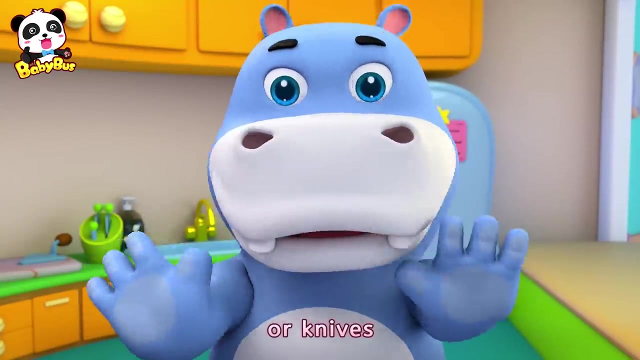 In the kitchen. be careful, It's dangerous. be careful, Be careful, Timmy. let's play in the living room, Uh-huh. Okay, Kids, please don't play in the kitchen. Bye, I got it. We shouldn't touch hot kettles, pots or knives. 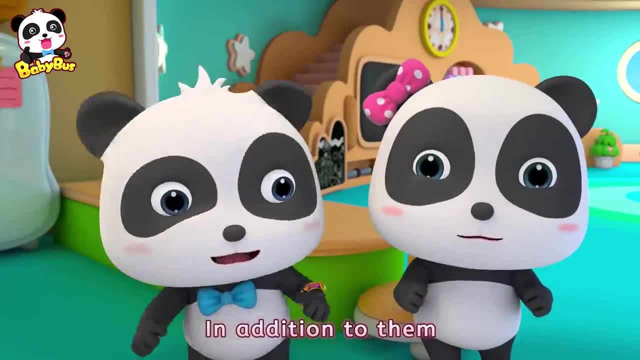 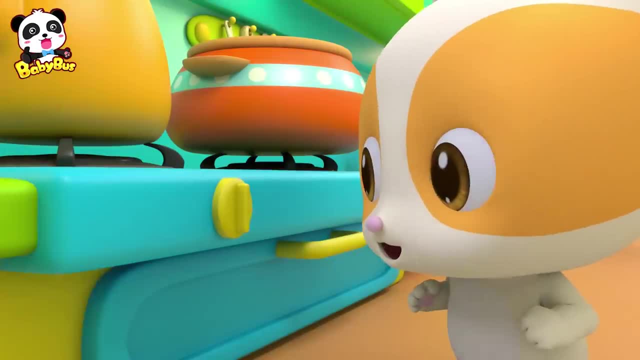 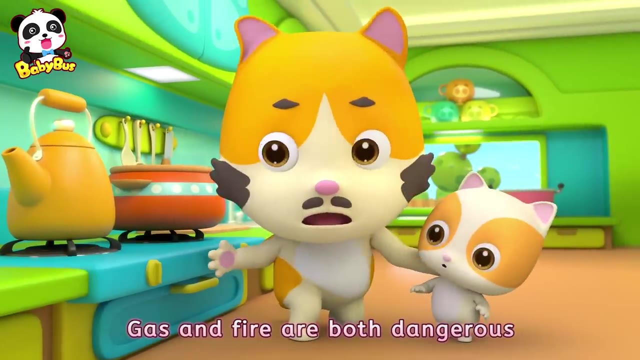 Right, Good job, Hank. In addition to them, there are some other things you need to be careful of. Let's take a look. Don't touch the gas stove switch. Gas and fire are both dangerous. Don't touch the microwave or oven when they're on. 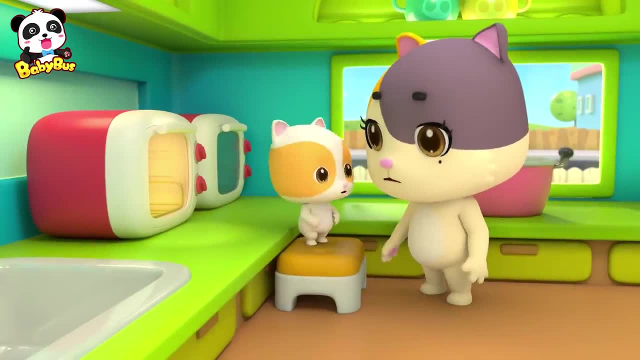 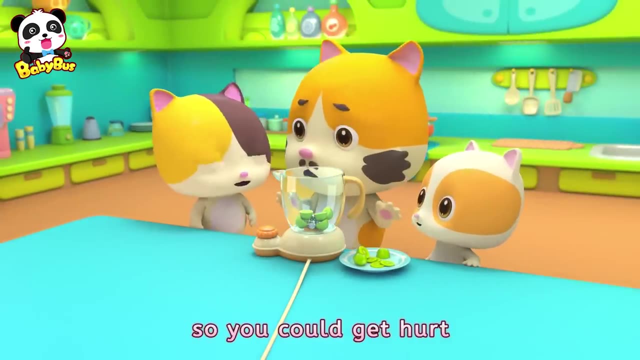 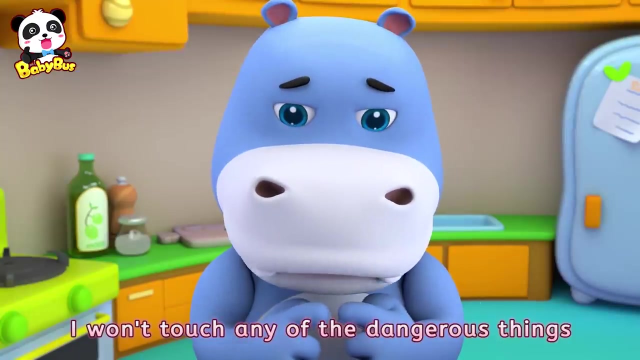 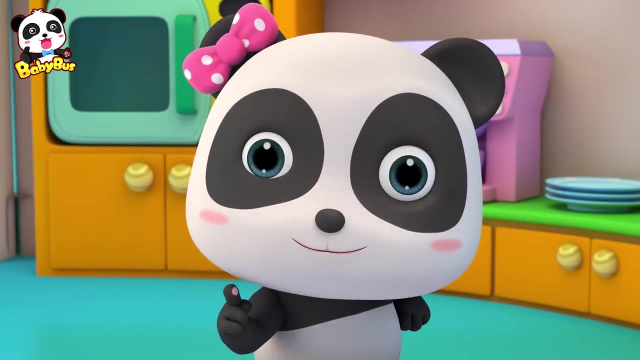 You could get burnt. Don't touch the blender. There is a sharp blade inside so you could get hurt. I won't touch any of the dangerous things in the kitchen. Kids, do you remember what we've learned today? Great, You've learned about safety. 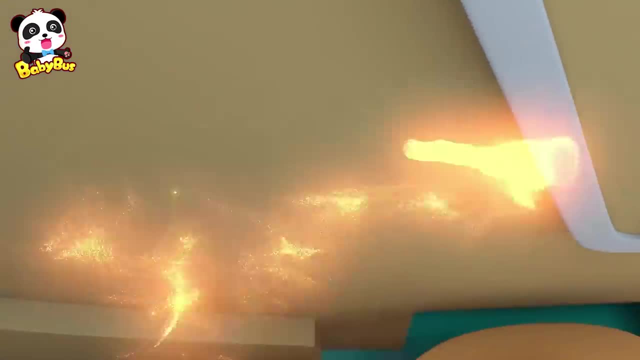 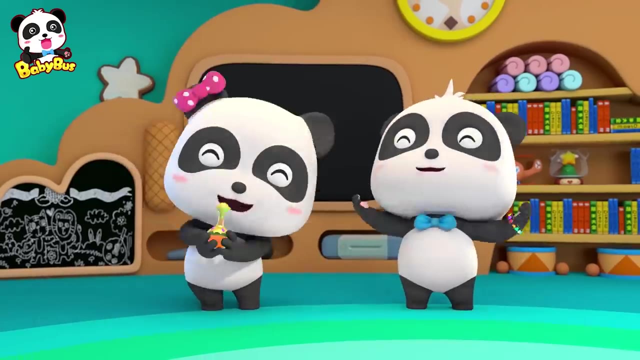 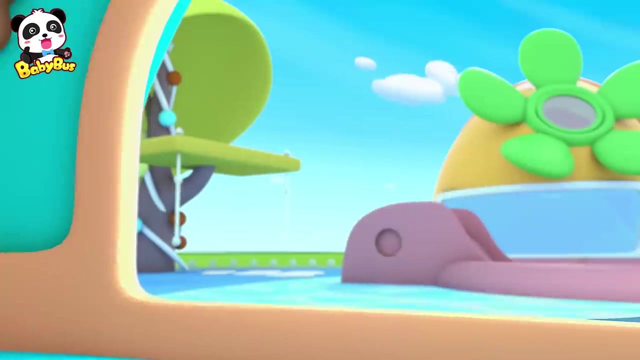 Wow, Wow, Yay, Yay, Yay, We've got a bottle of magic potion. Oh no, They've got a magic potion.